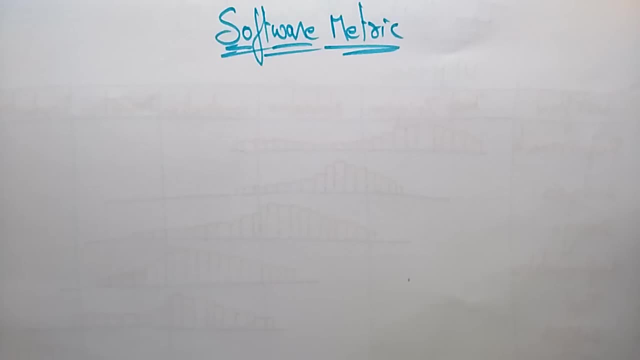 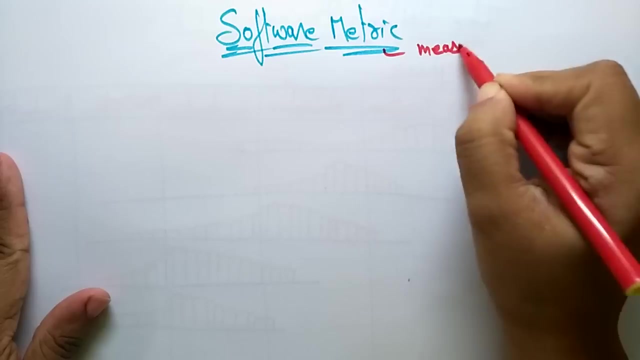 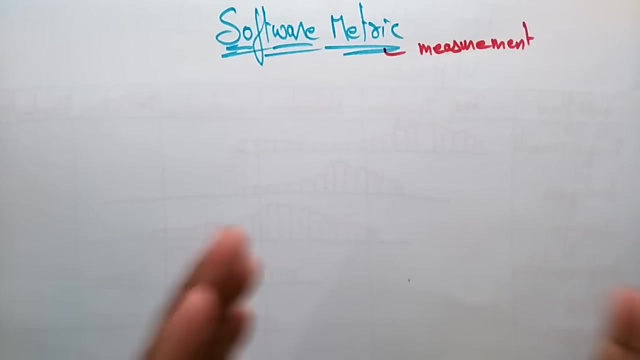 Hi students. coming to the next topic, that is, a software metric. So what is a software metric? A metric is nothing, but we call it as a measurement. It's just a measurement. So we will get a doubt how we can measure a software. A software is nothing, but it is a series of code. it's a line of code. So how we are going to measure the software and how we are going to give some systematic code to the customer. 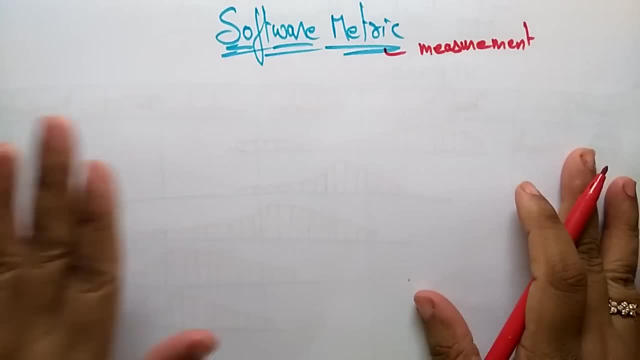 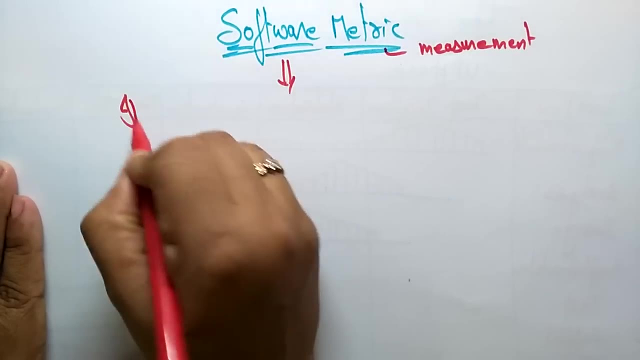 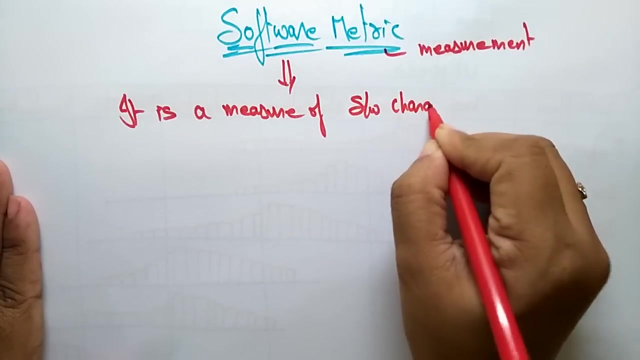 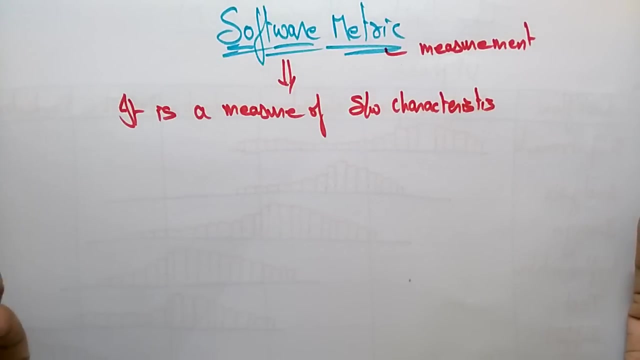 So now let us see. what is this exactly? the software metric was A. software metric is a measure of software characteristics. It is a measure of software characteristics. So what are those characteristics of software? It means the time it takes to execute the program. It means the quality of the software, the quantity that we are using, the resource that we are using, that everything comes under the characteristics. 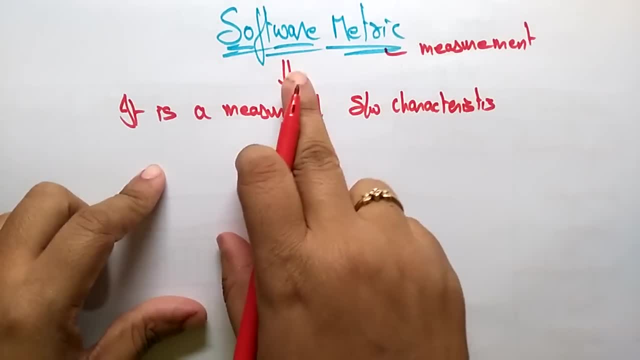 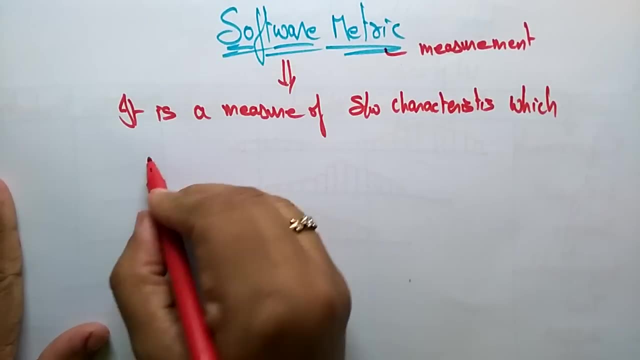 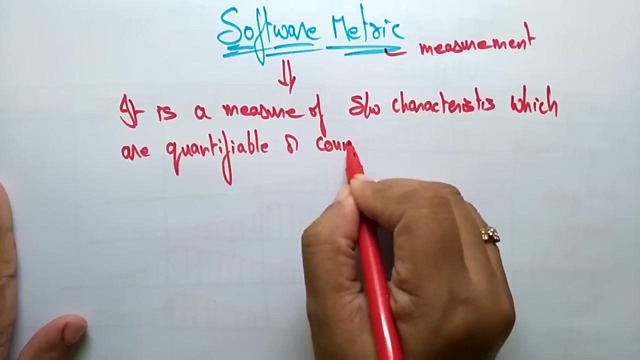 So we are measuring those characteristics that you call it as a software metric. A software metric is a measure of software characteristics which are quantifiable or countable. So we have to measure only the quantifiable and the quantable things that are present in the software. 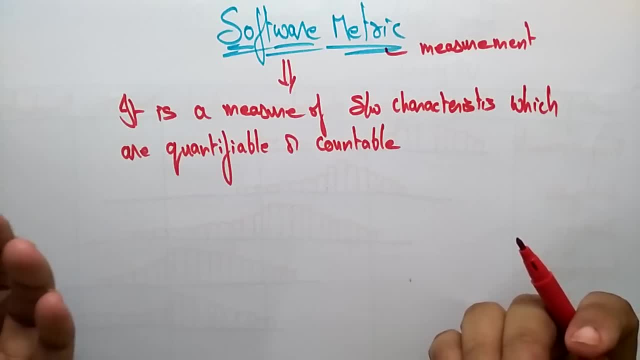 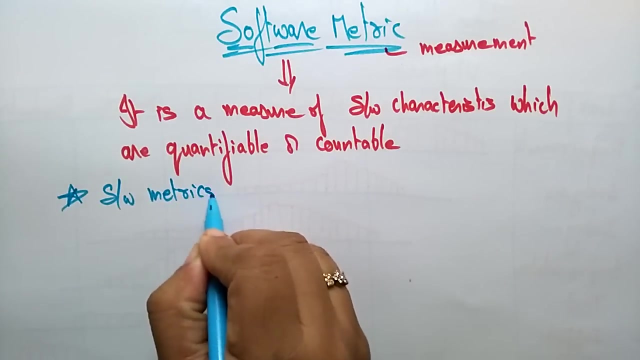 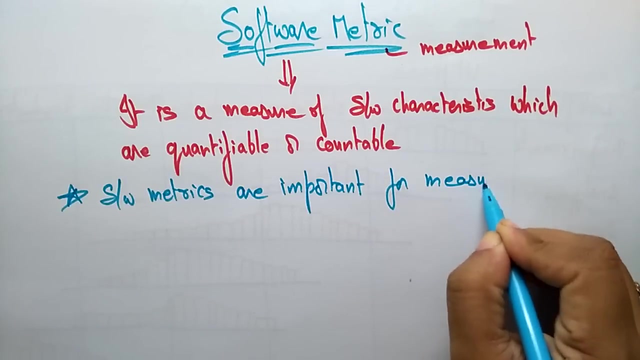 So if you are using some resource to develop a software, you have to calculate those characteristics, Those items also. That comes under the software metric. So a software metrics are important for measuring. The main thing is: the software metrics are important, Important for measuring, For measuring what? So measuring software performance? 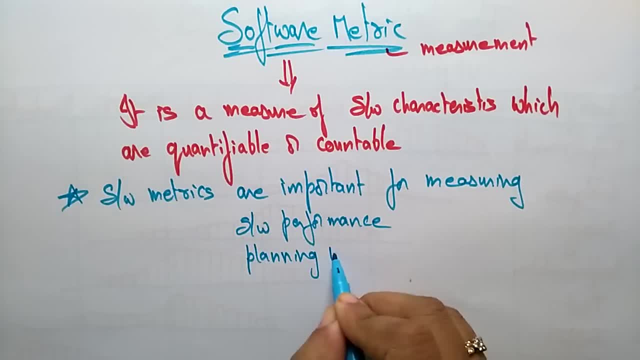 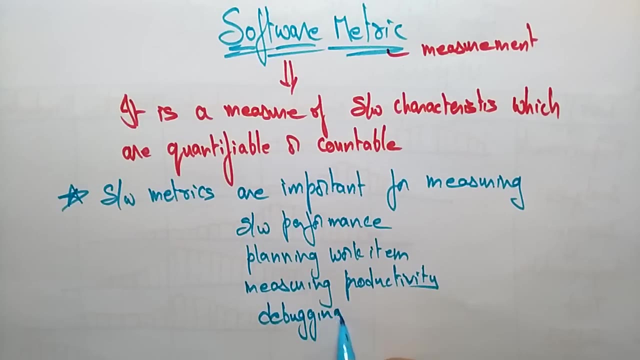 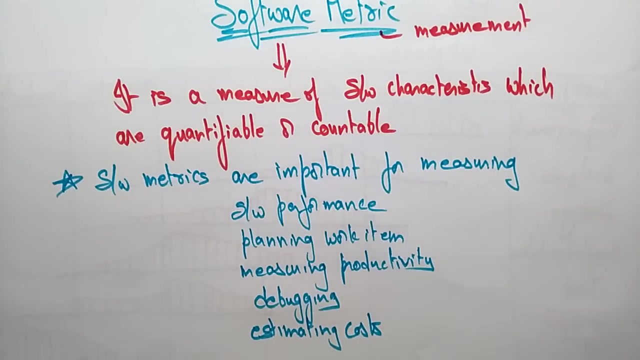 Software performance planning, work items and Measuring productivities. Measuring productivity, Debugging And estimating cost, Estimating cost, and So these are all the different measuring items that we came across in the software. So whatever the software you have taken, So if you want to measure the software, you have to consider these important measuring points. 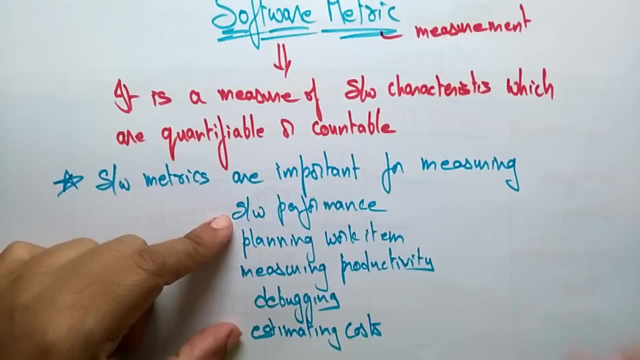 So you have to check the software performance, You have to measure the software performance. So what is the performance of the software that you are using? and the planning work items and measuring productivity, Debugging, estimating cost. so all these can helpful, important for measuring the software metrics. 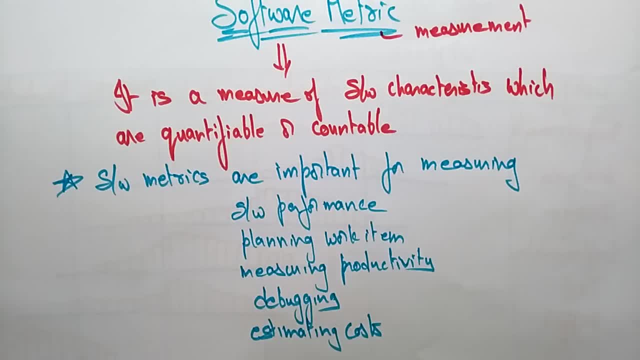 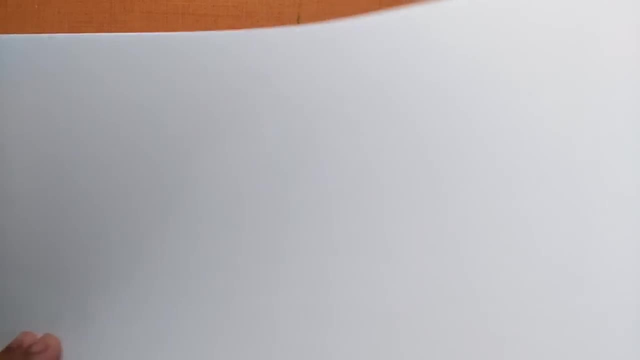 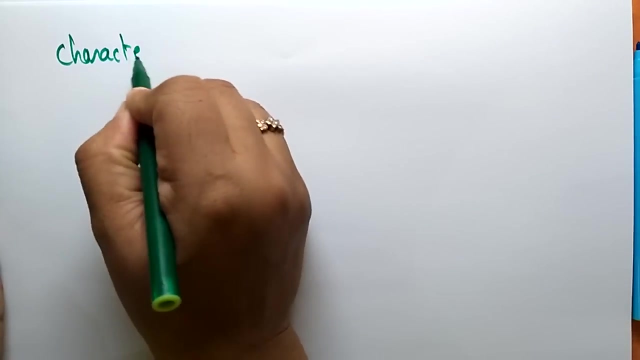 So, and also these components is valuable for both Developers and development team leaders. So the main thing Of software metrics is a valuable component for both developers and development team leaders. Now let us see the different characteristics that are present, that are in software metrics. The characteristics of software metrics. 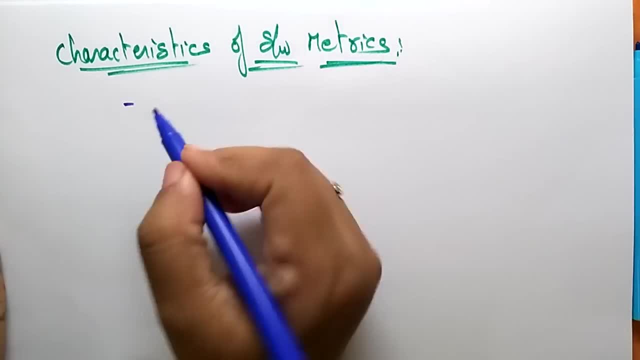 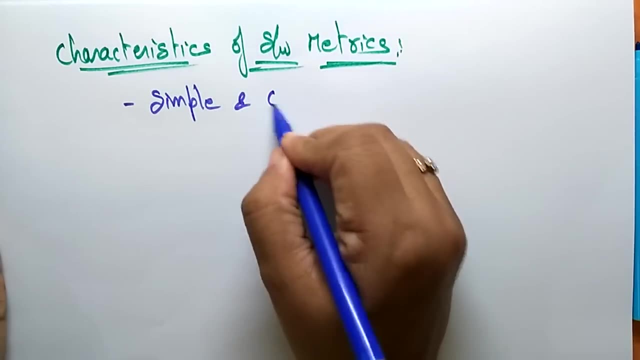 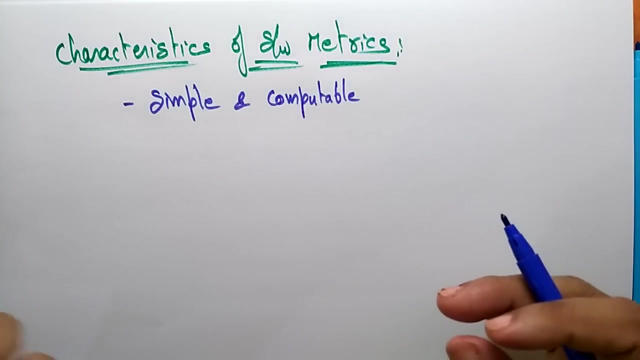 So what are the characteristics of software and metrics? so, first thing, it is simple and Computable. we can easily calculate the This software metrics only for the small lines of code. It's so you have to think if it is a your project, if your lines of code, if your program is small. 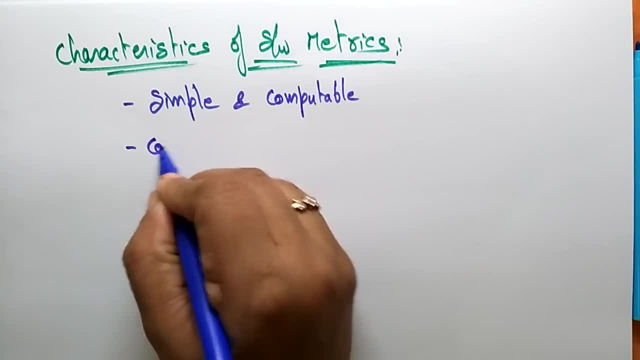 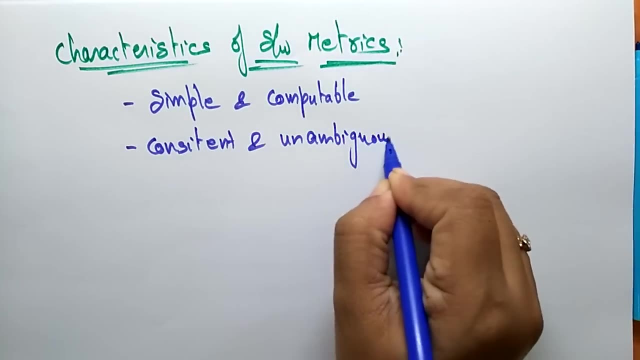 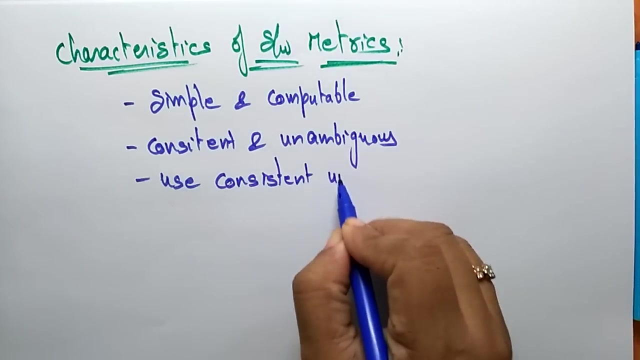 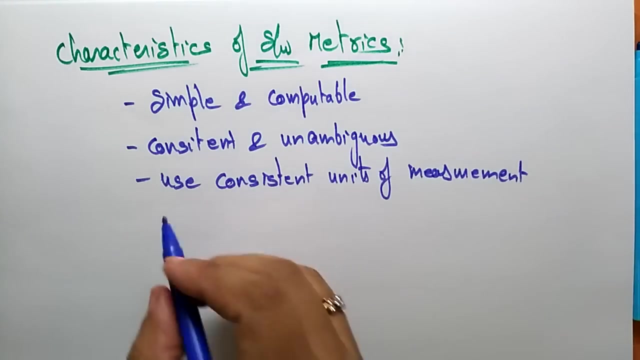 Then it is simple and computable, easily Consistent and Unambiguous. and Another characteristics: use consistent unit. Use consistent units of measurement. And it is independent of programming language. It's not dependent on means. for any type of programming language You can calculate the software metrics. So that's why we call it, as this software metric is an independent 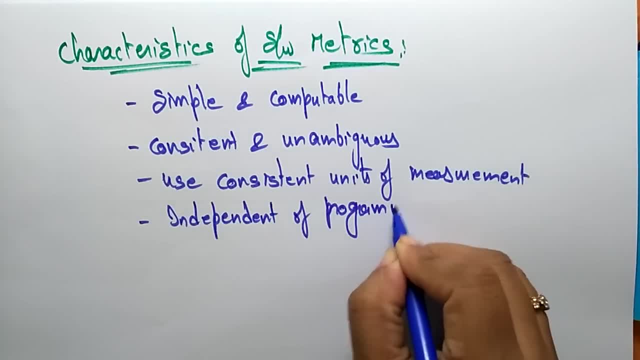 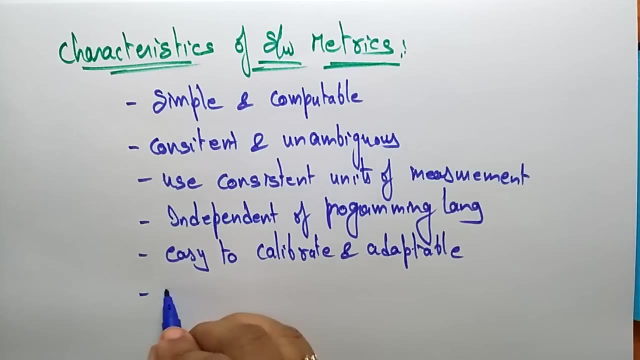 independent of programming language. and It is independent of programming language and It is easy to calibrate and adaptable And it is easy and cost effective to obtain- also Easy and cost effective to obtain. So these are all the different characteristics of software matrix. Thank you.